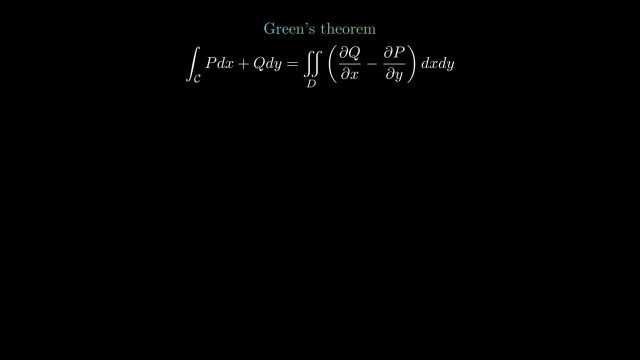 where p and q are functions of two variables, is given by the double integral over the region it bounds, which we've denoted by d, of partial q, partial x minus partial p, partial y of dx, dy. Now to have some intuition and actually understand what Green's theorem is saying, let's recall the fundamental. 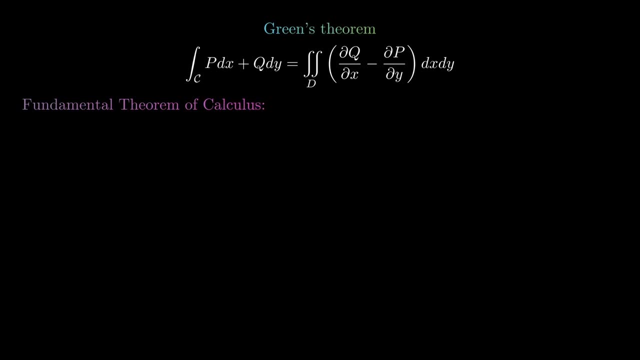 theorem of calculus that we learnt in kindergarten. So the formulation I'm going to take here is that the integral of a to b of f prime of x, dx is equal to f of b minus f of a. So if we look at the graph of f prime of x, the fundamental theorem of calculus tells: 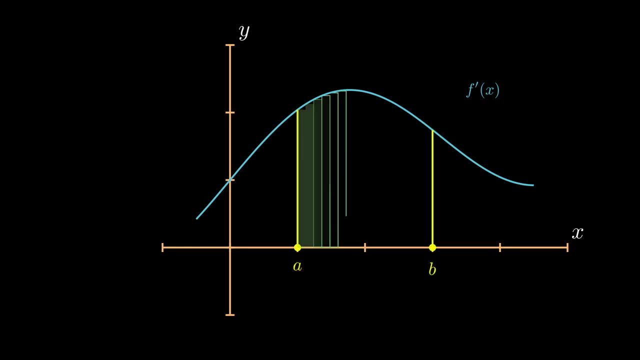 us that if we take two points, a and b, then the area underneath this graph is determined by the value of another function, namely f, at these boundary points alone. Now, a priori, we need to know every point between a and b to determine the area. but the fundamental theorem of calculus 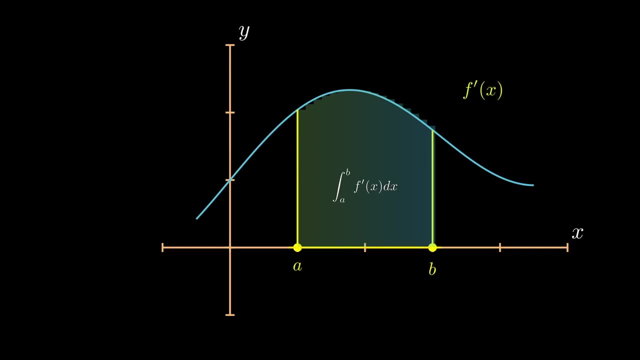 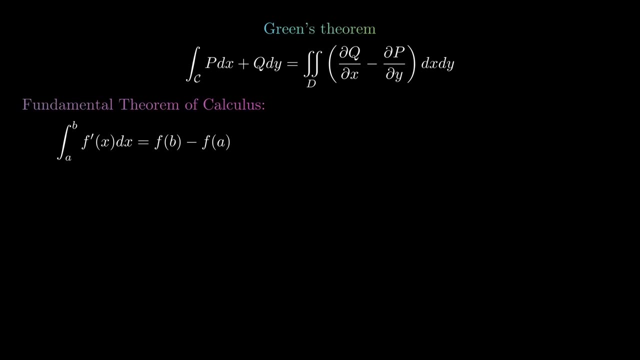 tells us that it's actually only determined by the values of a separate function, namely its antiderivative at the end points. Now to get further insight on the fundamental theorem of calculus, what we'll do is we'll rewrite the integral from a to b of f, prime of x, dx as the 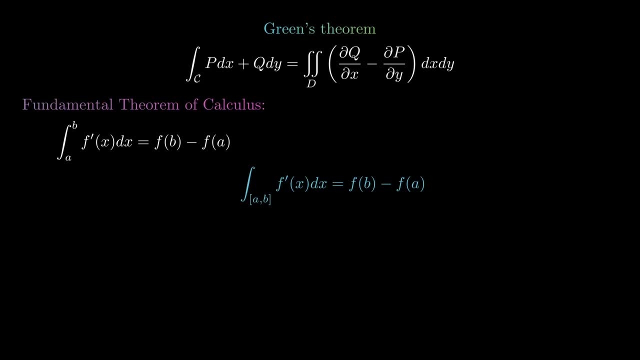 integral over the closed interval: a, b, f, prime of x, dx. For us this is going to be the same, and what we can do is we can also write f, prime of x, as df, dx. and what we can also do is write f, prime of x, as df, and we can also write a, b as the boundary of the closed interval: a, b, So to: 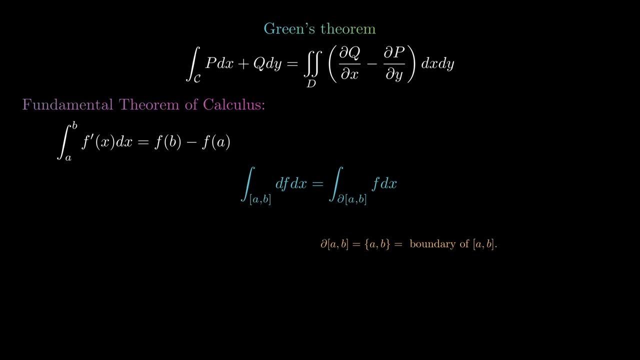 denote the boundary of a set, we use this partial symbol, so the set containing only the elements a- b, by partial of the closed interval a b. So now what the fundamental theorem of calculus says is that the integral over the closed interval a, b of df, dx is equal to the integral over the 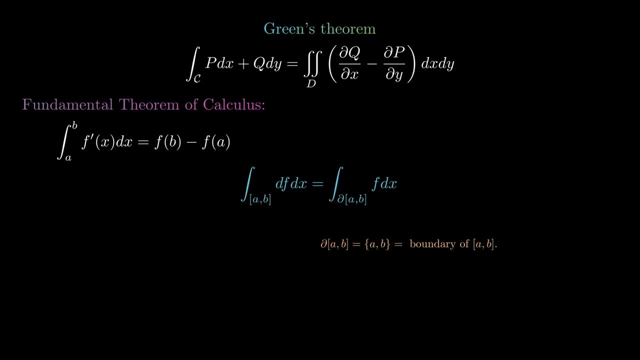 boundary of the closed interval of a, b, of f, dx. Now, just to make this subsequent remark more transparent, what we can do is it can actually replace df with partial f, since we're only dealing in the one variable situation. this is all equivalent, and so we've written the fundamental. 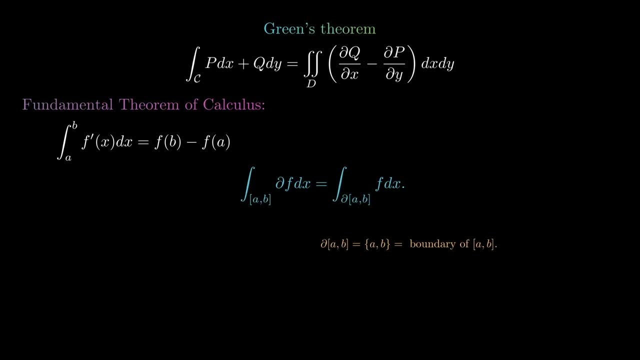 theorem of calculus, as the integral over the closed interval a- b of partial f? dx is equal to partial of the closed set a- b, in other words, the boundary of the closed interval a, b of f? dx. From this way that we've written the fundamental theorem of calculus, it's clear that integrals are: 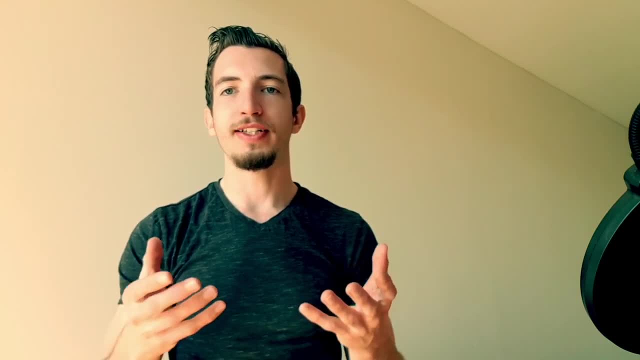 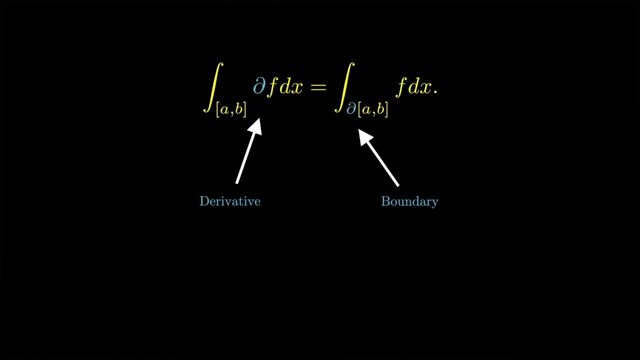 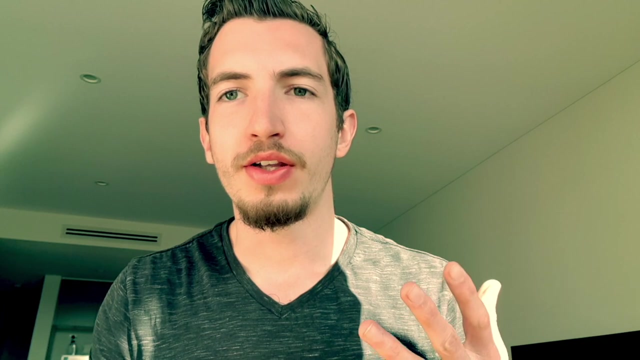 not necessarily the opposite of derivatives. What's happening is that the opposite of the derivative is actually the boundary of the region of integration. So the way in which this discussion that we've had so far is formalized is through what's referred to as duram cohomology. This is a subject within differential geometry that is covered within 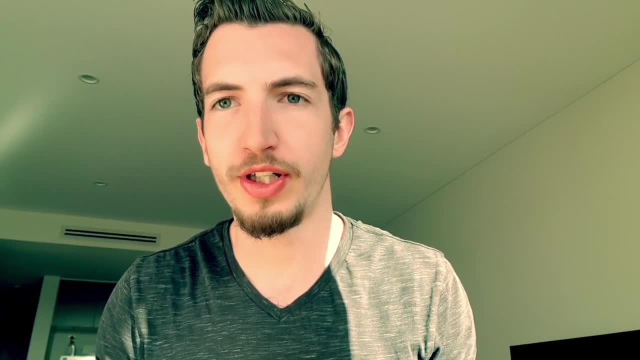 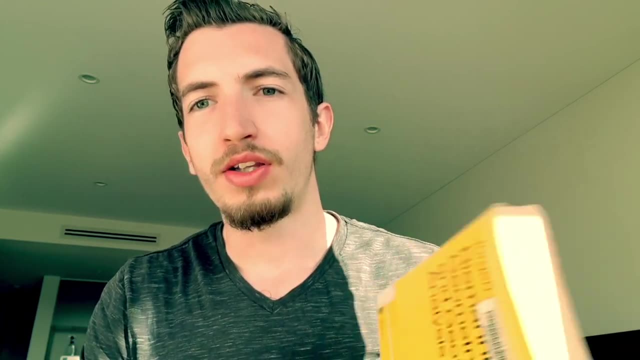 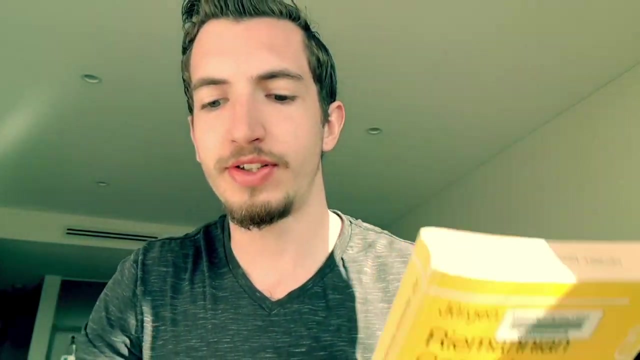 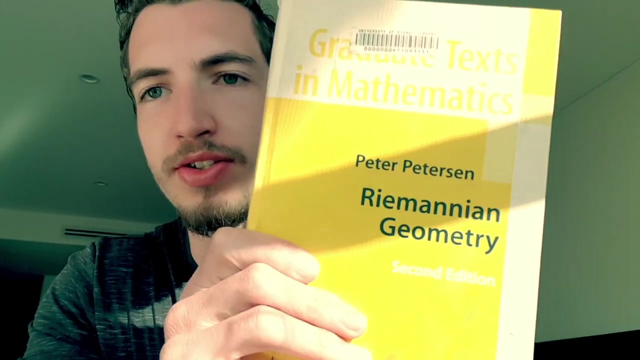 any standard text on romanian geometry or differential geometry, albeit it's quite an advanced concept subject to typically a graduate course. This can be found, for example, in Yost's romanian geometry and geometric analysis, or my favorite book on the subject, which is Peter Peterson's romanian geometry, the second edition. These are excellent books which 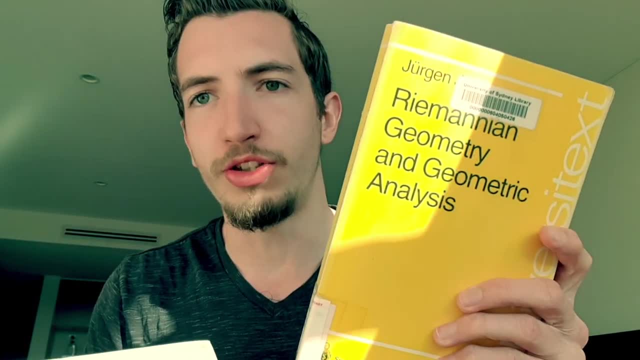 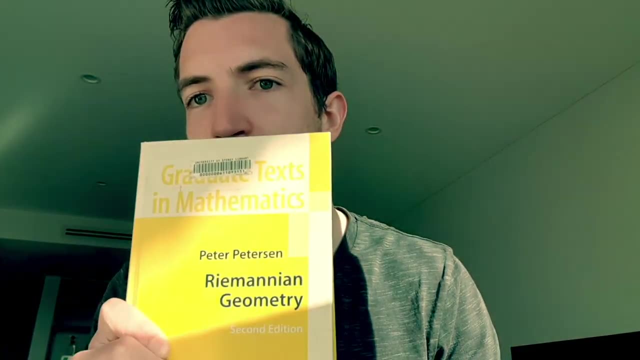 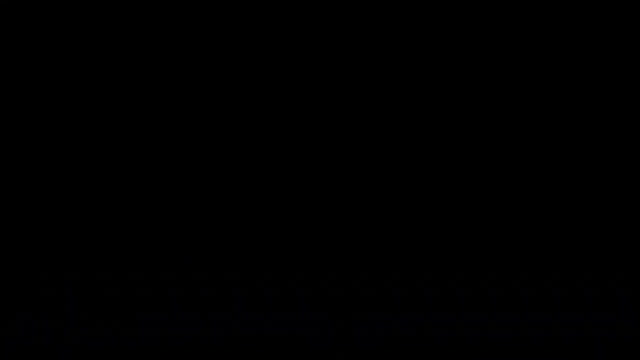 I would highly recommend. I initially learned romanian geometry from Yost's book under Ben Andrews and then, as a graduate student, I worked through and continue to work through Peter Peterson's romanian geometry book To continue this extension of the fundamental theorem of calculus in a hope to get something out of it. I'm going to show you how to do that in a moment. 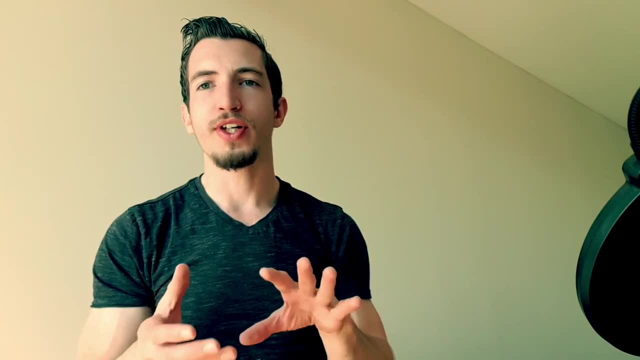 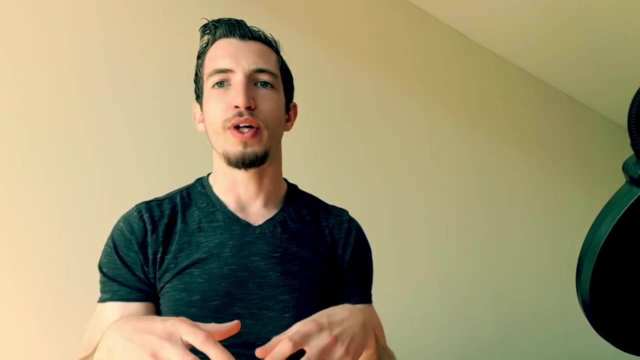 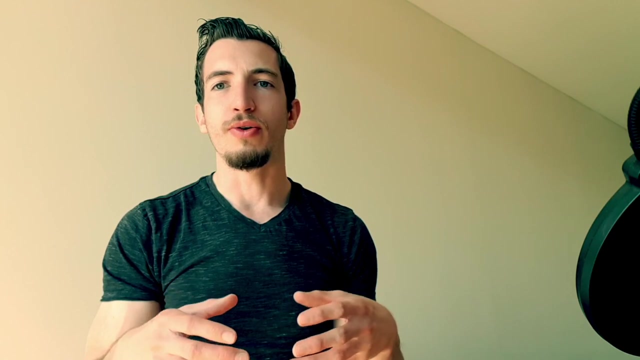 Inside, on Green's theorem. what we'll now do is ask the question of how can we formulate area, the notion of area, this abstract idea, into an operation that we can perform on vectors or something, or some type of object we're familiar with, in order to get a language that's actually. 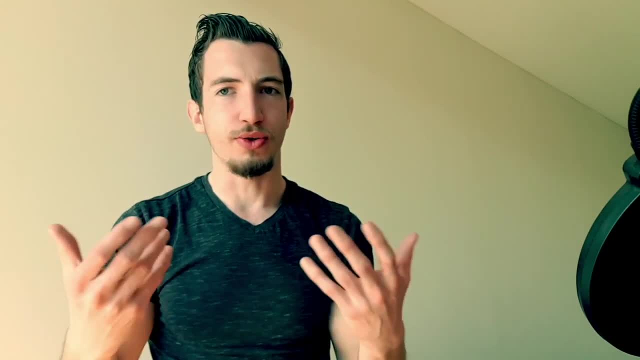 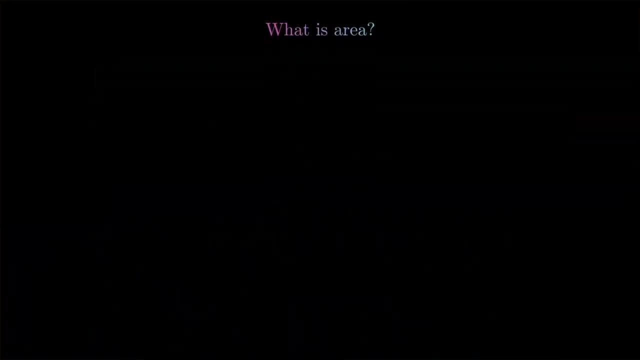 fruitful. So we want to develop a language on vectors or on some type of objects that furnish an understanding of what area is. So let's restrict our consideration to vectors. So let's consider the vector v, which is the vector 1, 2, and the vector u, which is given by 2, y. 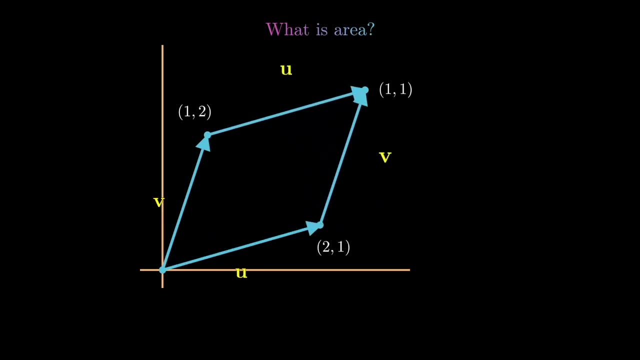 What we can, of course, do is translate v to the end point of u and u to the end point of v and form this parallelogram. Now, of course, from kindergarten linear algebra we know that the area of this parallelogram is just going to be given by the determinant of the matrix, whose 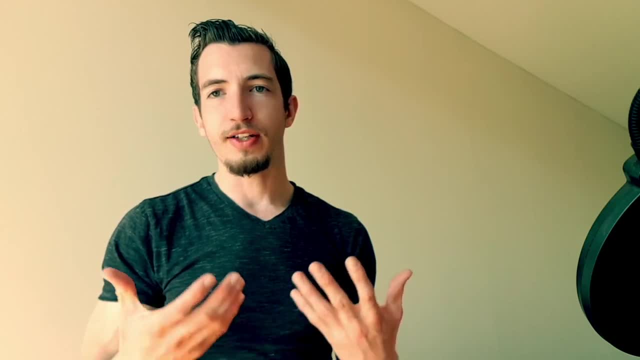 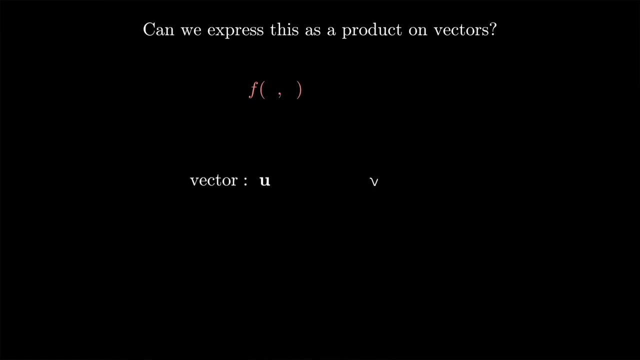 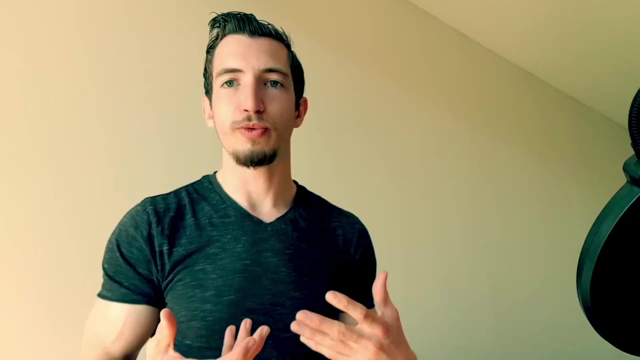 vector is given by u and v, But we'd like to express that in an operation. We would like to know whether we can actually construct an operation on vectors such that if we take a vector u, take a vector v, apply this operation. it gives us the area of the parallelogram. 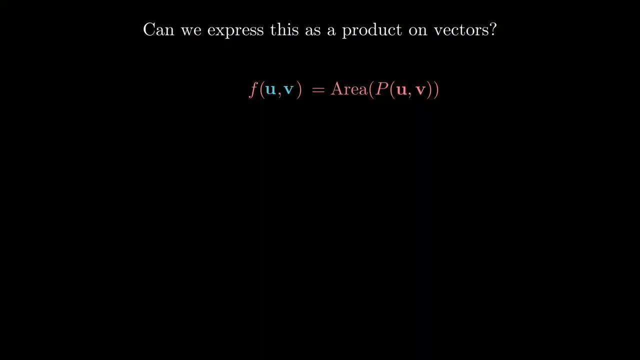 This will be an important key step in the development of this formalism. So let's assume we have such an operation, We'll denote it by this wedge symbol here, So by u, wedge v In the area of the parallelogram formed by u and v. 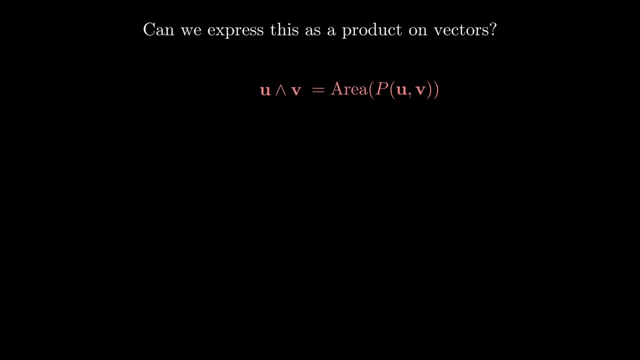 To get an understanding of exactly what properties this operation would have, what we'll do is we'll write u as a, i plus b j and v as c, i plus d j. Now the wedge of u and v is then just a: i b j. wedge c: i plus d j. 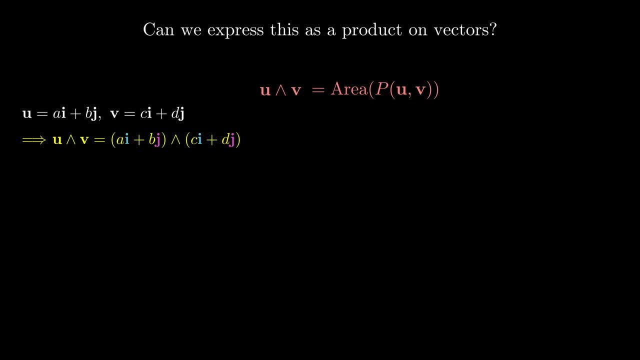 We'll assume that it's distributive, so we can foil it out in the sense that we'll now have a- i wedge c i plus d j plus b- j wedge c- i plus d j, And then this would further expand to ac- i wedge i. 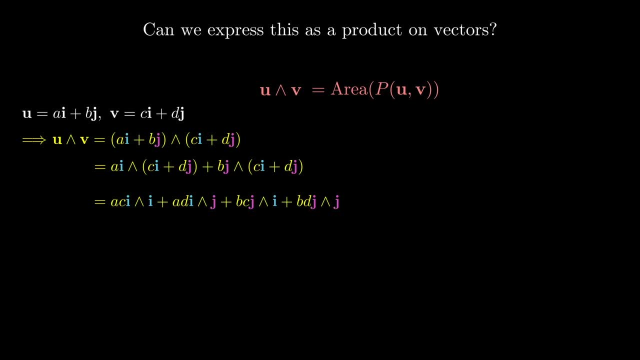 plus ad. i wedge j plus b c j wedge i plus b d, j wedge j. Now, of course, i wedge i is the area of the parallelogram formed with i in itself, and j wedge j is the area of the parallelogram formed with j in itself. 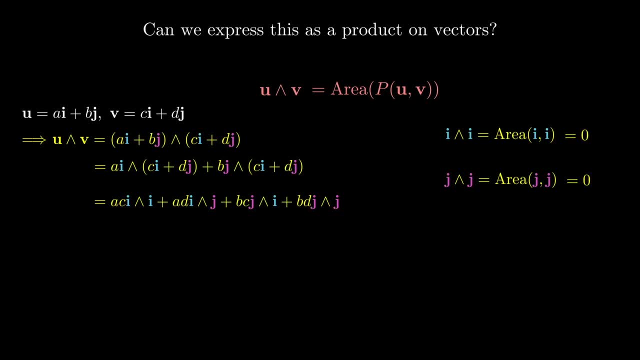 the area of a line which, of course, is zero. So now what we can do from what we've just calculated is that in this u wedge v calculation, the first term and the last term, which are the i wedge i and j wedge j terms, are both zero. What we're now left with, therefore, is that u wedge v is ad i wedge j. 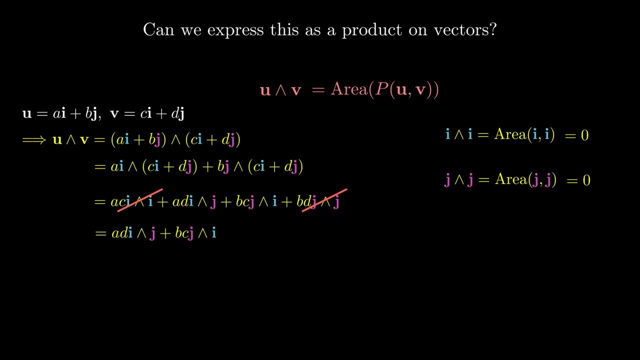 plus bc: j wedge i. And now we want to understand how does this wedge operation behave if we switch the order? So what is the difference between i wedge j and j wedge i? So we'll recall that i wedge i and j wedge j. well, they're areas of lines, so they're going to be zero And, in particular, I can: 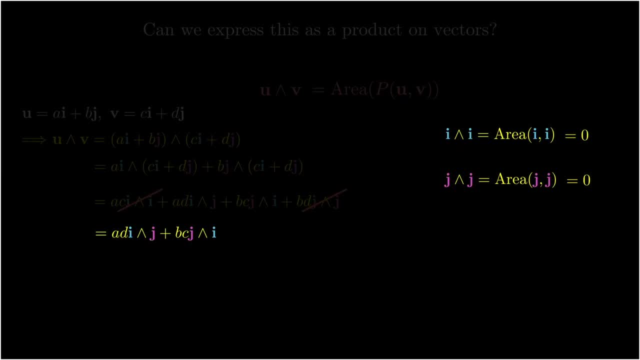 consider the parallelogram formed with i plus j and itself. Again, that's just going to be the area of a line, so it will also be zero. So we have that zero is equal to i plus j, wedge i plus j. Expanding this out, we get i wedge i plus. 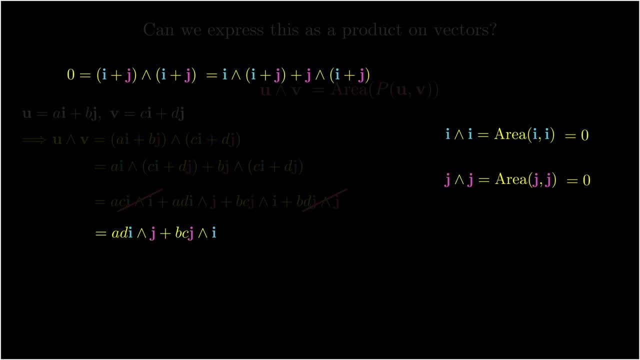 j plus j wedge i plus j, which we further expand to i wedge i plus i wedge j plus j wedge i plus j wedge j. This is exactly what we did before. Again, the first term and the last term will cancel and we see that zero is equal to i wedge j plus j wedge i. In other words, we get the following: 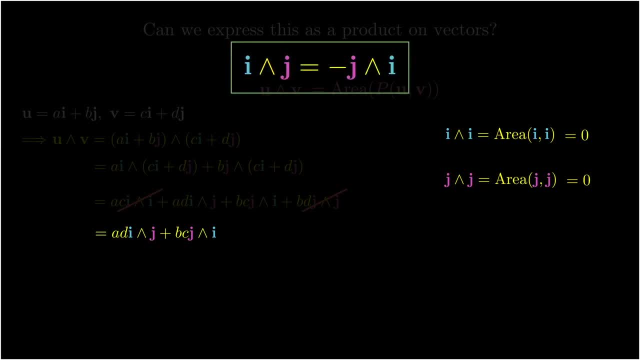 anti-symmetric property, which is that i wedge j is equal to minus j wedge i. So when we switch the order with respect to this wedge operation, we pick up a minus sign. So now, if we return to our calculation here, namely the u wedge v is ad i wedge j plus bc j wedge i. Then 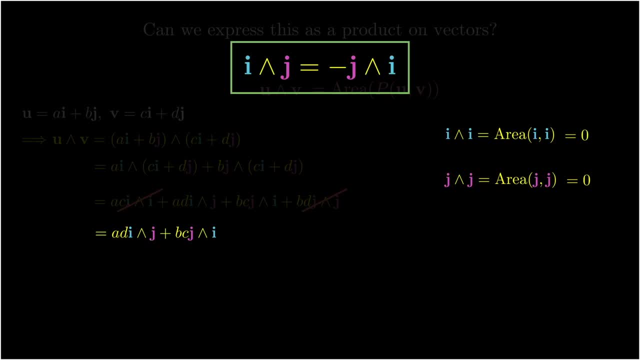 switching the order expressing everything in terms of i wedge j, we get ad. i wedge j minus bc. i wedge j, which, of course, we can just write as ad minus bc. i wedge j, which may surprise you or may not, but that's exactly what the determinant of a two by two matrix is, if the matrix is a, b, c, d, So this wedge. 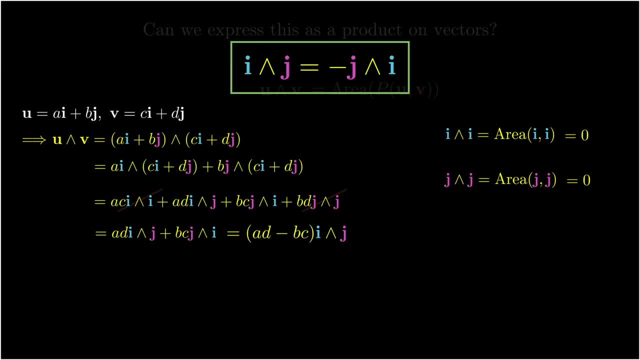 operation is exactly what we wanted. It gives us the area of the parallelogram of the vectors, where the vectors are columns of this matrix. So this wedge operation gives us exactly what we wanted. We want the area of the parallelogram formed by the vectors u and v. Now this operation on vectors. 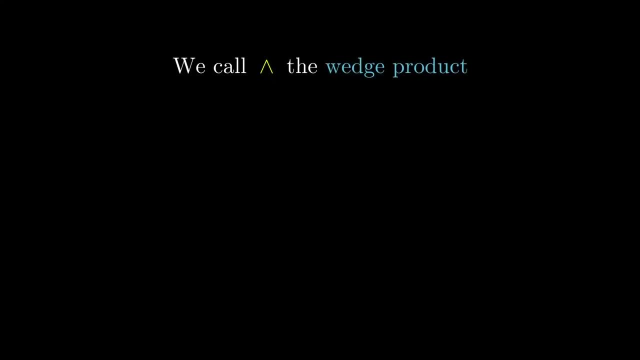 is well known. It's it's known as the wedge operation. It's known as the wedge operation. So the defining properties of the wedge product are that if we wedge something with itself, we get zero Again. that's because it's the area of a line, The parallelogram formed by a vector in itself. 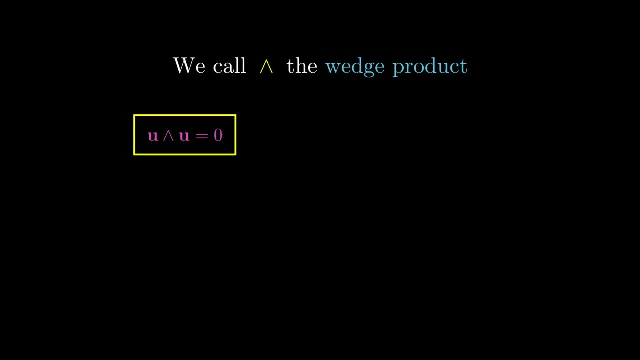 is going to be a line with area zero And it has the following anti-symmetry property, which is that u wedge v is minus b wedge u. Okay, so let's see how this new language tells us anything new or gives us any insight into. 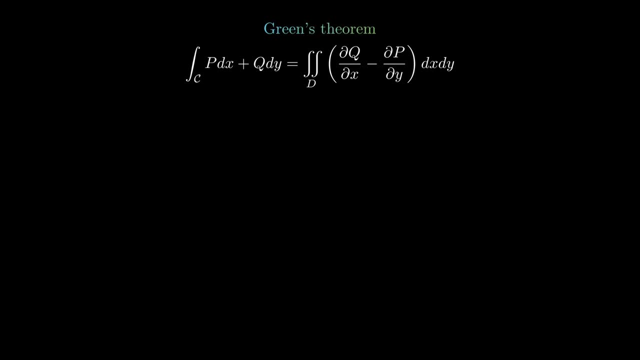 what we're going to be able to do. So what we're going to do is we're going to use the Green's theorem. So recall the Green's theorem again: is the line integral over a closed loop c of pdx plus qdy. 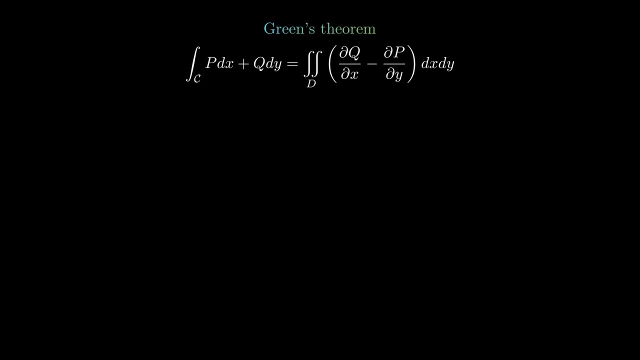 That's the double integral over the region and bounds of partial q, partial x minus partial p, partial y, dx, dy. What we're going to do is we're going to write omega as pdx plus qdy And we want to compute the derivative of omega, which we denote by d omega. Now, that's going to be the derivative. 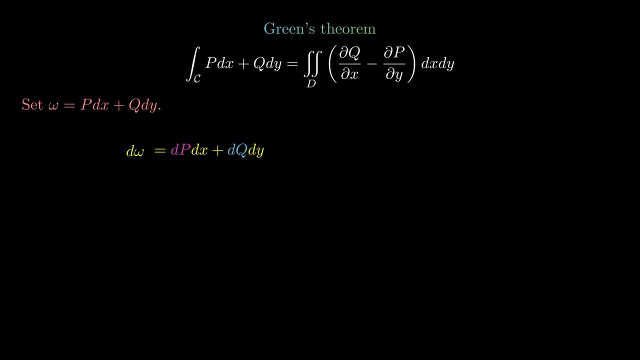 of the first function, dx, plus the derivative of the second function, dq, dy. Now we're dealing with a function of two variables and we're going to use the following definition of the derivative, which is that if we have some function f, then df is partial f, partial x, dx plus partial f, partial y. 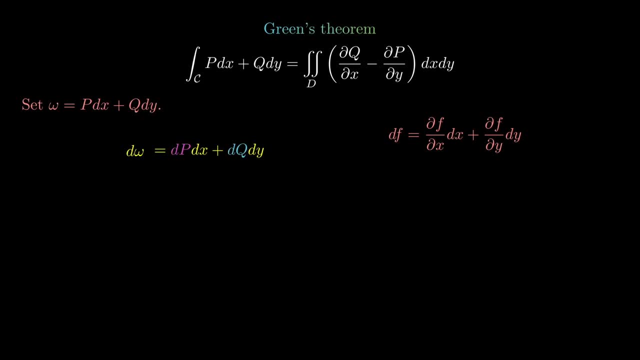 dy. This is well known to be what's referred to as the exterior derivative, but the name is not important here. So if we use this definition of the derivative, what we see is that dp is the derivative of the first function. dp is going to be partial p, partial x, dx plus partial p, partial y. 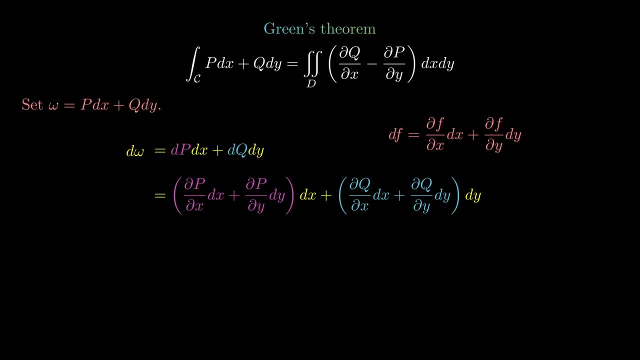 dy, And then we have the dx plus. now dq is partial q, partial x dx plus partial q, partial y dy, And then we'll have dy at the end. Now, what's implicit here is that there are actually going to be wedges here. 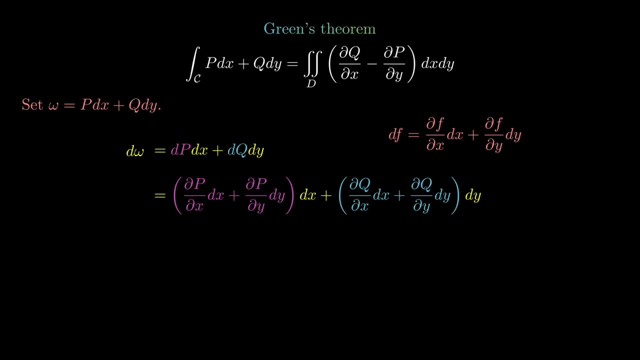 So whenever we write dx, dy or dx, dx, implicit in that is that there is a wedge. These are referred to as covectors and covectors are covectors and covectors are covectors and covectors are covectors, Which can just be thought of as vectors for this discussion, And we're pairing them in such a way. 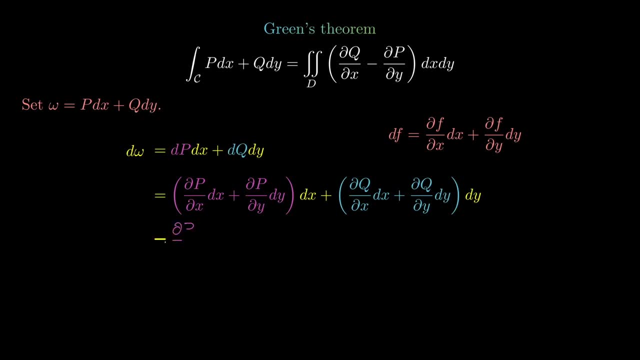 that we get area. That's what integrals yield. So what we have is partial p, partial x dx- wedge dx, plus partial p, partial y dy- wedge dx. Then similarly partial q, partial x dx- wedge dy, plus partial q, partial y dy- wedge dy. This is just distributing the previous line. Now recall that. 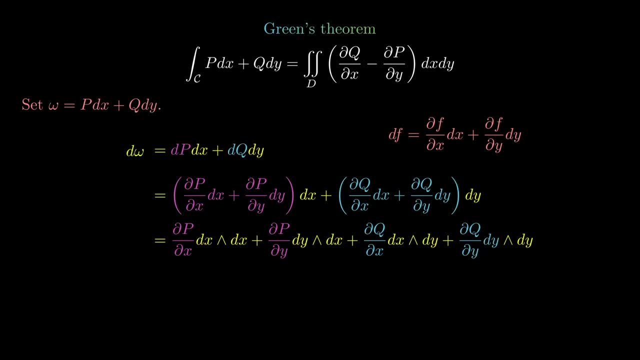 if we wedge something with itself, that will give us the area of a line and that'll be zero. So immediately we see that the first term and the last term here- partial p, partial x and partial q, partial y terms- both vanish And we're left with partial p, partial y, dy, wedge dx plus partial q. 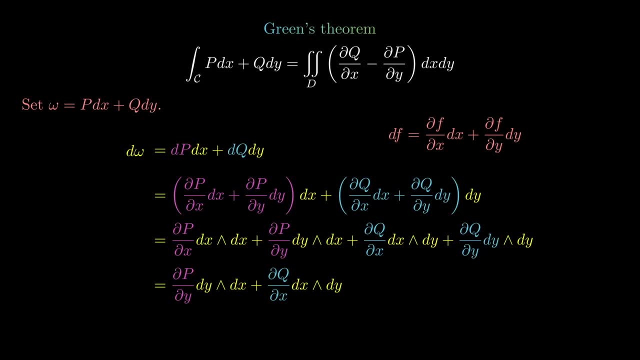 partial x dx, wedge dy. Now, the other property of the wedge product was the anti-symmetry. So if we switched the order of what we were wedging, we would pick up a minus sign In particular. what we see, is that what we? 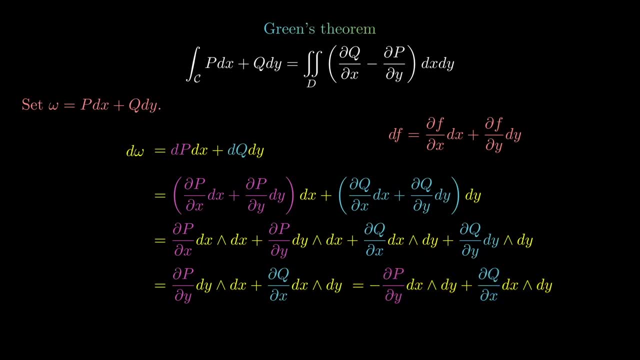 have here is minus partial p, partial y dx wedge dy, plus partial q, partial x dx wedge dy. And then of course we can combine this and just write this as partial q, partial x, minus partial p, partial y of dx wedge dy. And if we compare this with Green's theorem, what we see is that the left-hand side is: 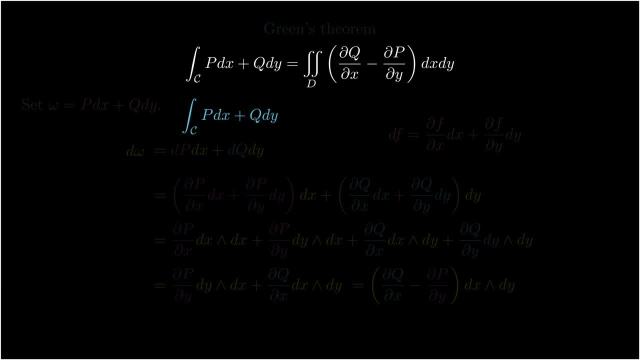 the integral over the boundary of d. So we can write c as partial d of omega And we can write the right-hand side, namely this double integral, as the integral over the entire region. you can keep the double integral notation, if you prefer, of d, omega. And what this right-hand side of Green's theorem is saying is that we 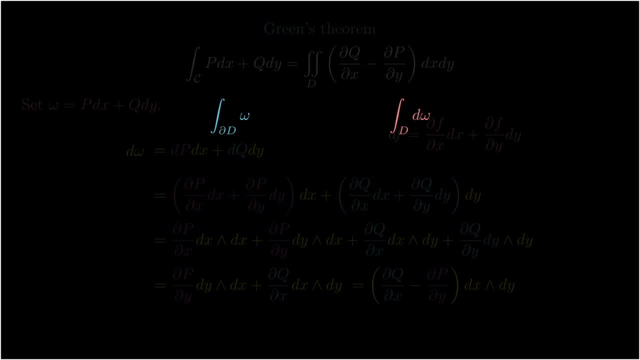 have the integral over the entire region of the derivative, And so, in particular, Green's theorem is saying that the integral over the boundary of omega is the integral over the entire region of d omega. When we write it like this, symbolically, we're only referring to: 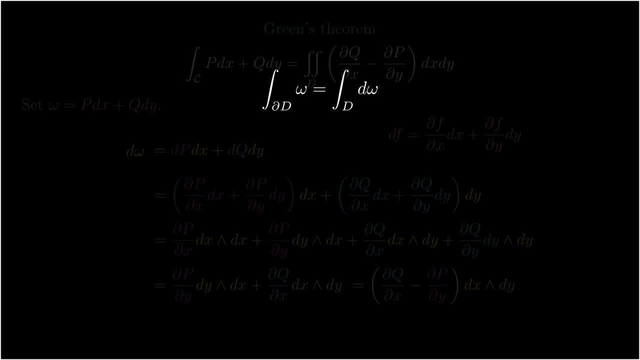 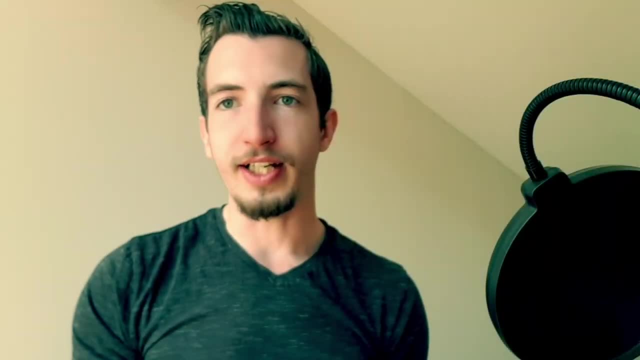 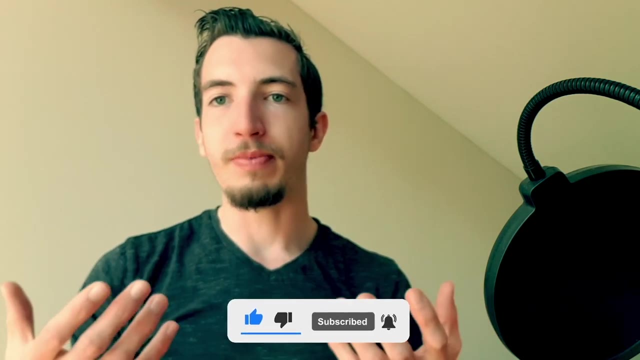 regions in the plane, but it holds in higher dimensions. This is in its full generality. it's referred to as Stoke's theorem. What I hope is being made clear at this point now is that Green's theorem, when expressed in this language, of wedge products, and in my opinion,